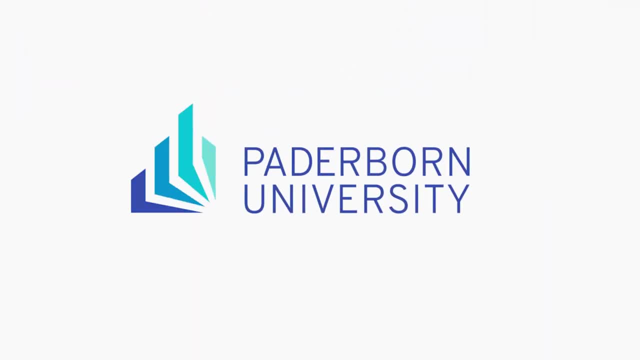 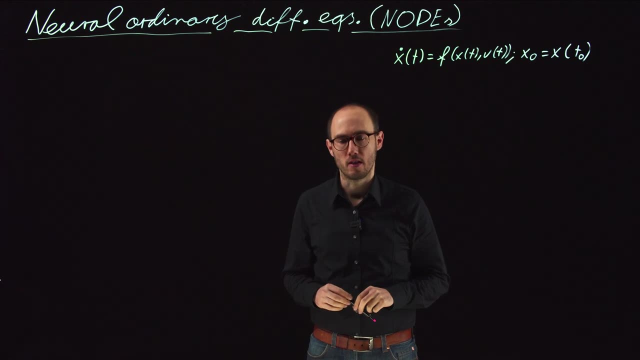 Hey everyone, in this video we are going to deepen our knowledge about nonlinear system identification and we will use the so-called neural ordinary differential equations, or so-called nodes. The use case of the nodes is that, again, we want to model a potentially nonlinear ODE. 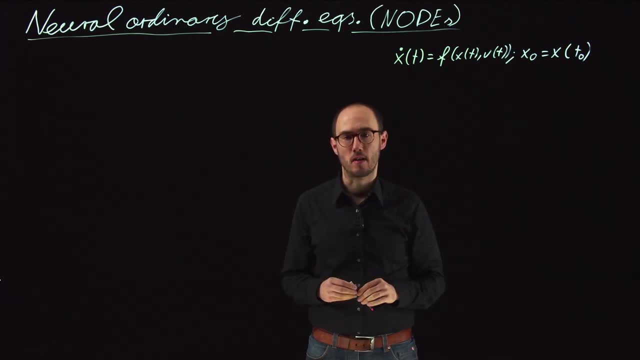 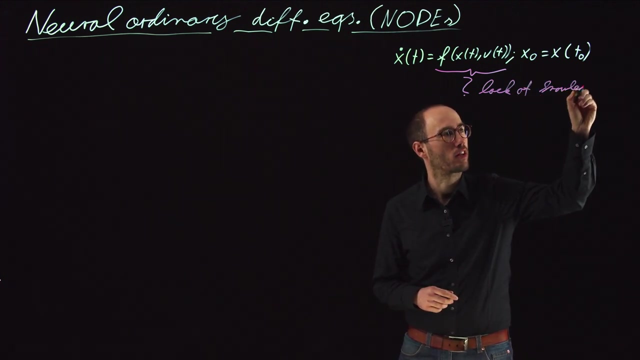 and in contrast to our previous videos where we did parameter identification, so where we have used structural knowledge on the system, we are now going to assume that we exactly lack this pre-knowledge. So we say that we have no knowledge of the system. structure Lack of knowledge. 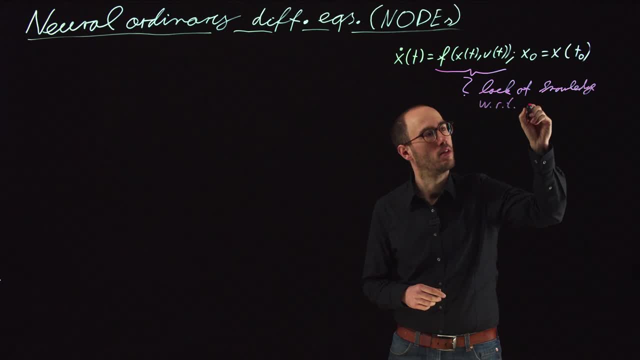 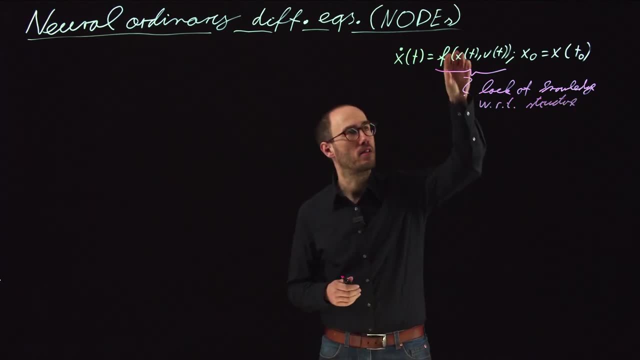 with respect to structure. So if we do not have specific insights like how this right-hand side of the ODE is internally structured, of course we normally also do not have the opportunity to model physical or interpretable parameters within this right-hand side. So we need not only to find some parameters. 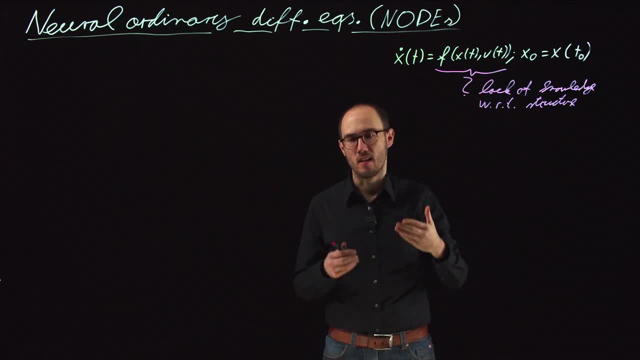 describing the right-hand side, but we also need to find the actual structure to represent it, And one way in order to do this is the so-called node approach. So what is the idea? The idea is quite straightforward: Instead of putting something in terms of parameters on the right-hand side, 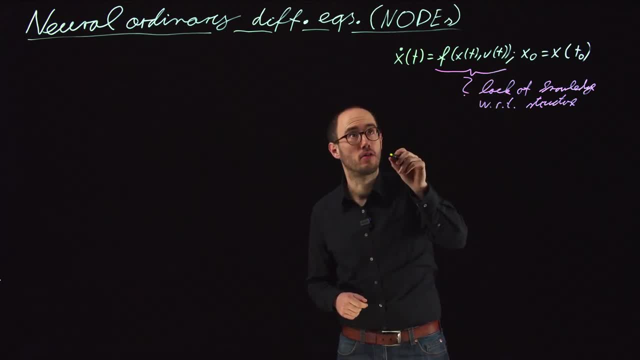 which are physical and interpretable. we take an artificial neural network, so an ANN with the inputs of x of n and x of n. So we take an artificial neural network, so an ANN, with the inputs of x of n and x of n. 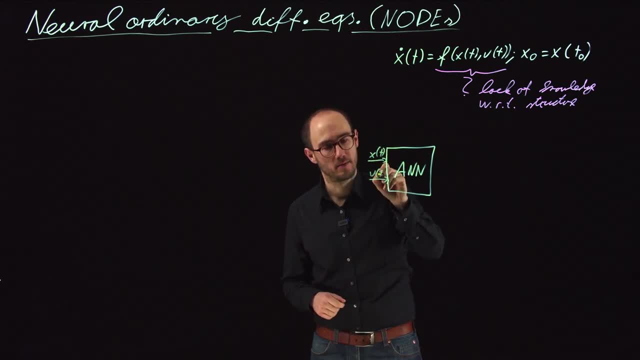 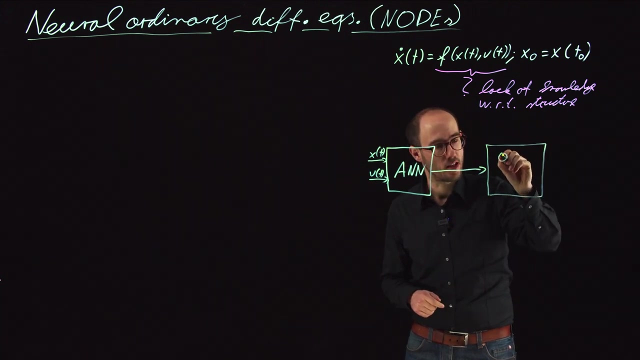 So the Christian is wavery, add parties. you have the so s here, the right hand side of the ODE, and the output of this ANN is then fed into an ODE representation plus ODE Solver. So that would be basically this entire structure plus one of the solvers which we have already discussed. 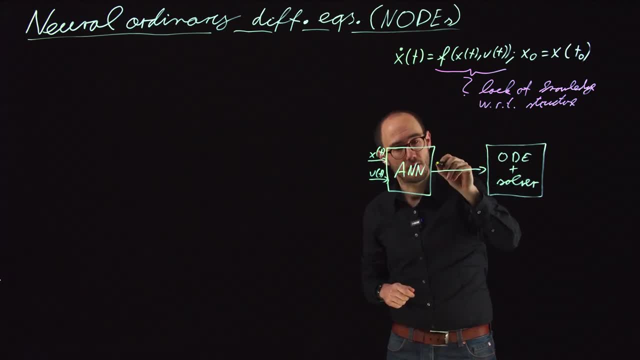 wrapping around that, and this output here of the ODE will be f hat, so an approximation of this right-hand side with some abstract or potentially abstract parameters, w, depending on x and u, and this will be x dot right. so representation of the right-hand side and if our ODE solver solves this, 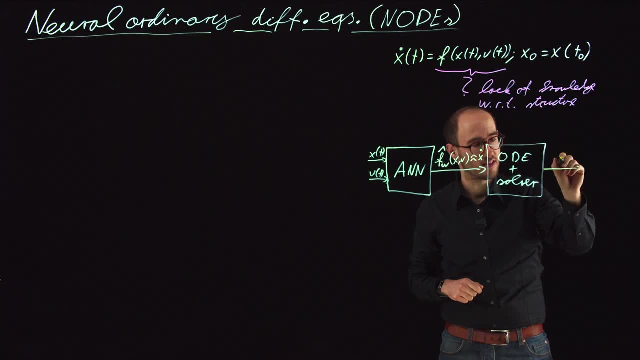 approximate right-hand side. what we of course get from that is x hat of t, so our representation of the time-based solution, and if we want to utilize that for simulation, we of course need to feed that back here into the input in order to have, let's say, a closed looped simulation which we can utilize in order. 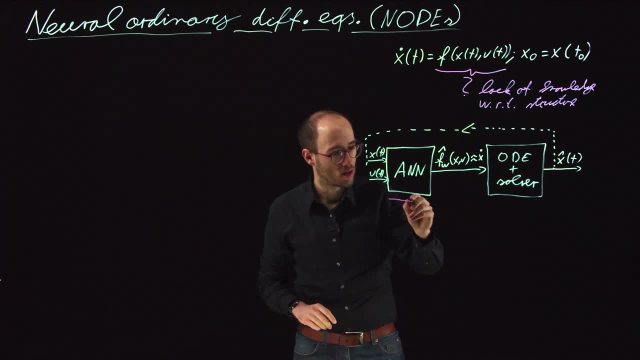 to solve the right-hand side and this combination of a and n- so absolutely abstract representation of the right-hand side- plus the ODE solver, is called the node approach Right. so formally this is just another optimization problem in terms of machine learning. so what we're going to do here is we want to minimize with 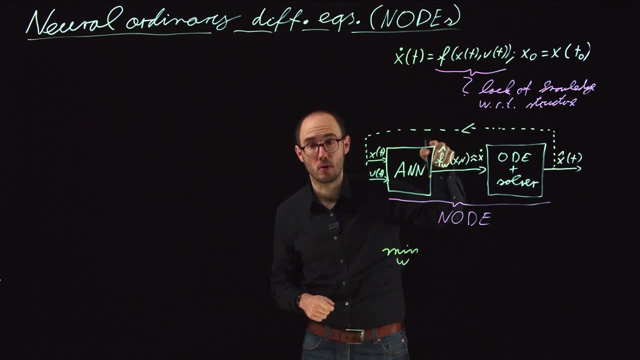 respect to the parameters w, representing this approximate right-hand side of our neural ODE, of a very classical logical function which we consider: the sum of k equals 1, up to n sampling points of x, of k, which is some sample ground truth data minus x hat of k, in the MSE kind of way. 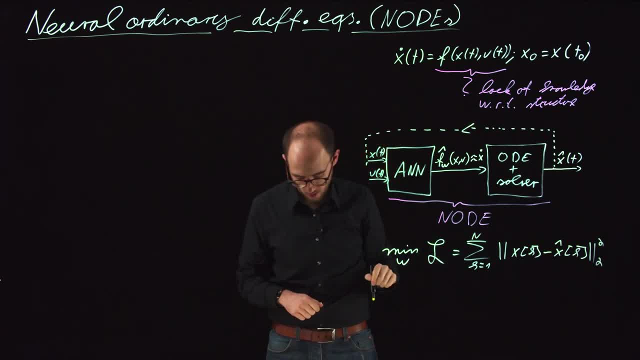 which is the output here of this right hand side, using the node approach, and this needs to be solved with. subject to x, hat dot is f, w, hat, x of hat and you and we do this on a time base. Tk is equal to k times Delta, T being some time. 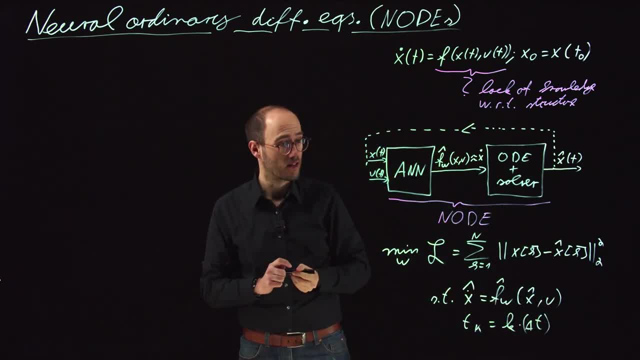 steps on which we actually evaluate this sample down situation just to see if it can be solved. this need to be solved with subject to x. hat at dot is f, w, hat X most probably cost function. So pretty much just another potentially non-linear optimization problem. 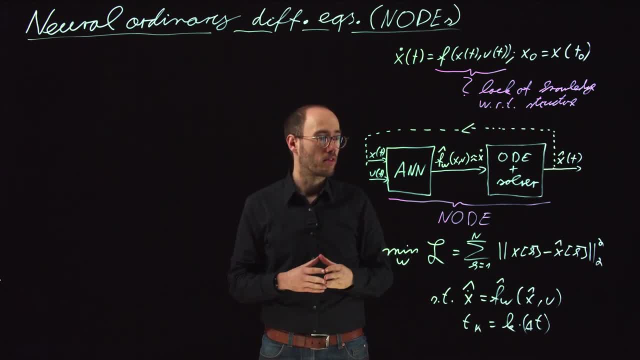 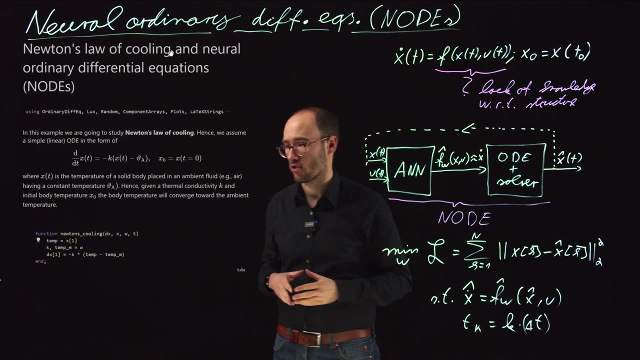 as we have already discussed that, the big new element of this approach is now that we do not assume any pre-knowledge about the right-hand side and we were represented by a general ANN, So let's get some intuition by that, by a practical implementation example. 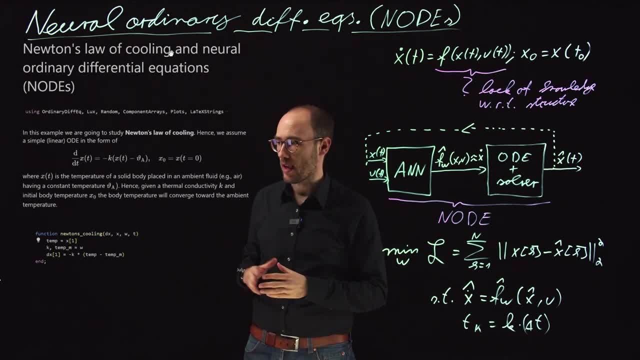 In this practical implementation example, we actually start with a very simple linear ODE as ground truth data in Newton's cooling law, which basically means that we just need to put in some temperature, ambient temperature, and we are modeling the temperature x of t of some solid metal, for example, being in an ambient airflow. So very simple ground truth problem and, of course, 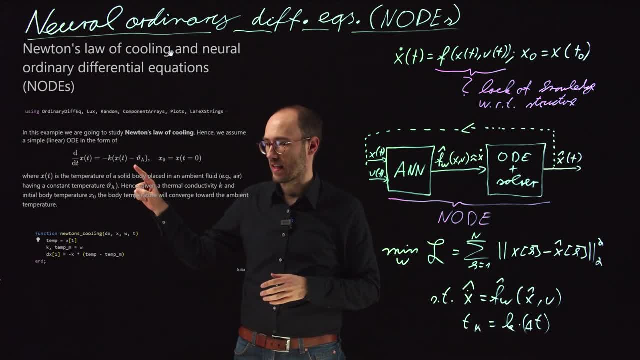 on the following: we do assume that we have a very simple ground truth problem, That we do not have, let's say, knowledge about the structure of the right-hand side. so we do not know that the right-hand side is such simple. We just utilize it in order to get some ground truth data. 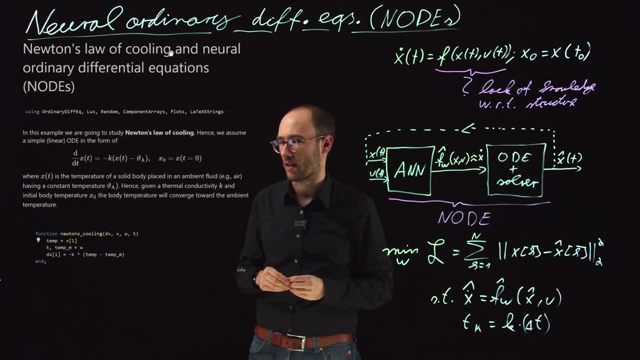 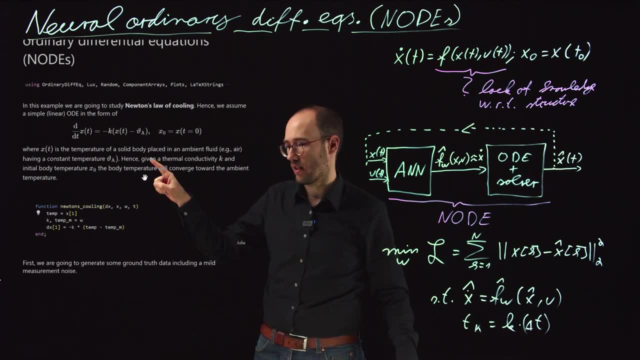 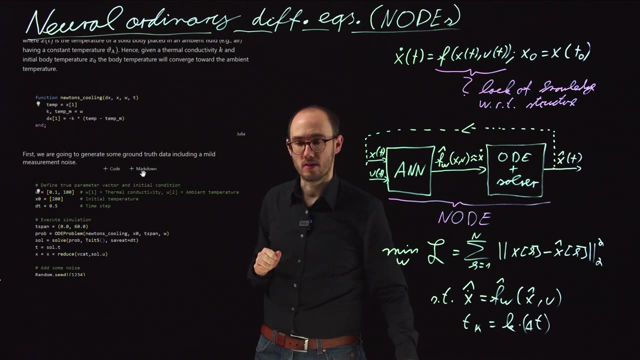 x of k first, and then we use the node approach trying to optimize it. So what do we do? We start with setting up the ODE in the function Newton's cooling very classically. Then we set up some general simulation parameters, put everything into. 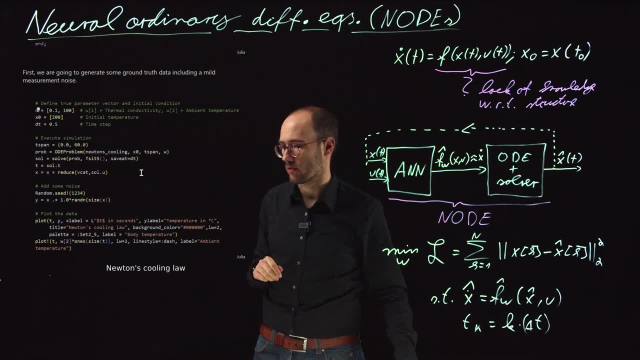 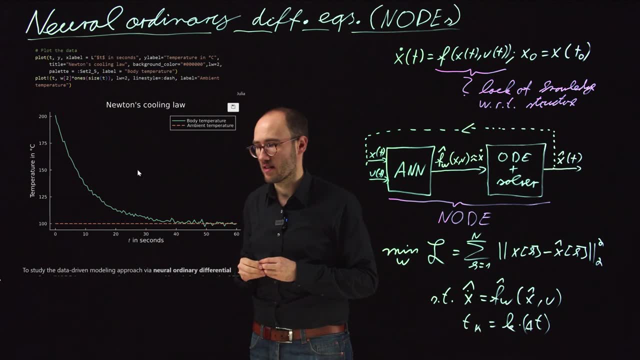 an ODE solver using the differential eq package from Julia and the ground truth system. response is as follows. So we assume that our metal element, which is sitting in just air, is heating up to 200 degrees celsius and we assume that the ambient temperature is 100 degrees celsius. 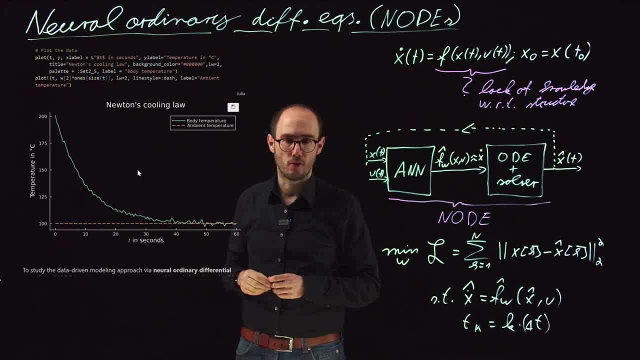 So what we see, including some measurement noise, is this first order decay of the temperature of this body, which is then approximately converging to the ambient temperature, which is to be expected given the Newton's cooling law. Okay, so this is our ground truth data. We know this greenish. 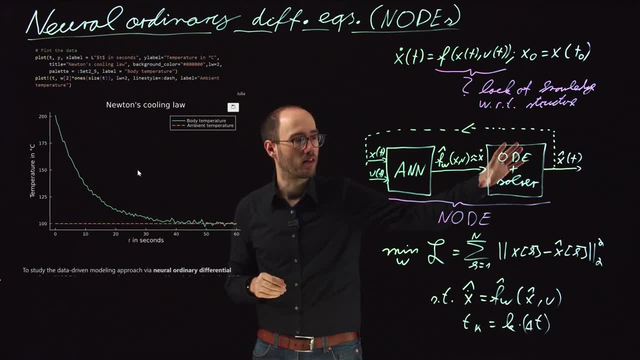 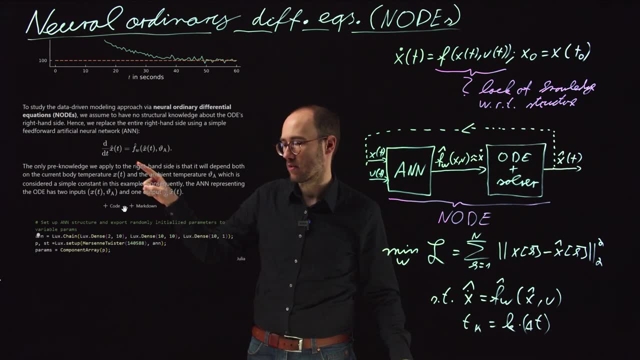 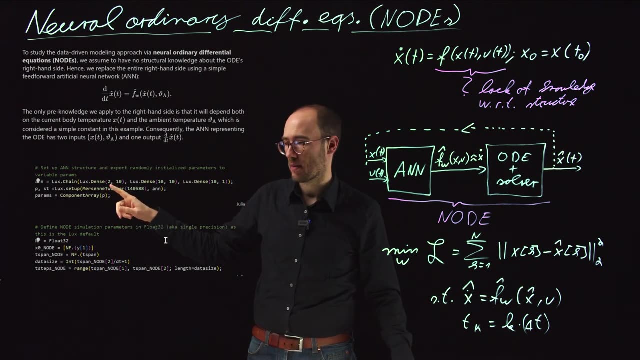 data trajectory, and now we are going to apply the node approach. So what do we need for that? So, first of all, we of course need some right-hand side, and this right-hand side in this, let's say, First attempt will be an artificial neural network using the lax package of Julia with two inputs. 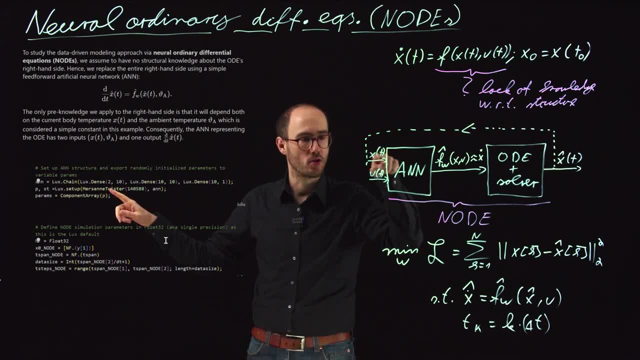 Why do we need two inputs? We need one for X of T, which is a scalar, and U of T, which is our ambient temperature, Which is another scalar. and we just do like a very simple, more or less randomly picked Neural network here, with one hidden layer not too big and the output layer, which is a scalar. 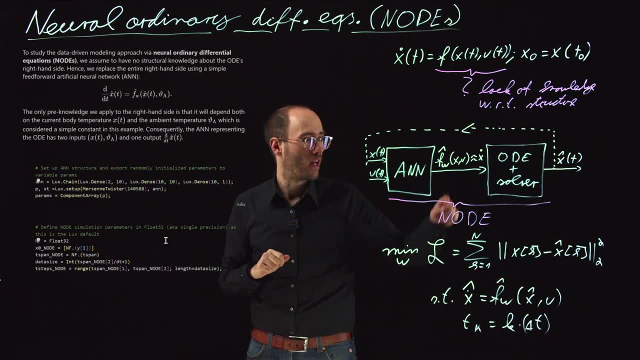 So this one here is basically the output dimension, And of course the ODE is a scalar ODE, so our output is just of dimension one. Okay, so a very simple neural network, nothing fancy here, more or less randomly picked. Then we need to configure the simulation of the ODE solver, of the node approach. 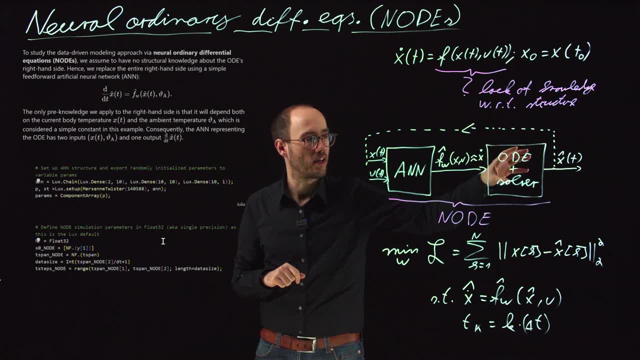 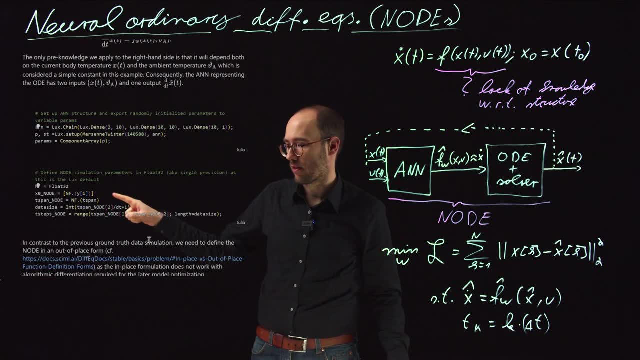 So we basically need to configure this right-hand side solver for the node training Which we do here on the part of the code and we do everything in single precision. so float32, in order to be compliant with the laxjl package, and order, in order to give have also a speedy simulation. 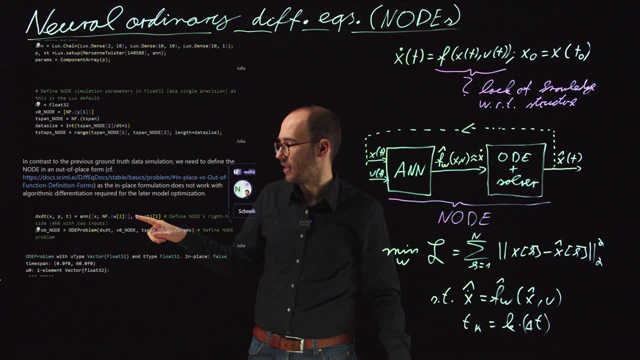 Then we put everything into the Solver, So we put here the ANN as the right-hand side of DXDT, right? So this is basically our ODE problem and we do not assume any further pre-knowledge. Then we have our ODE problem, and for this 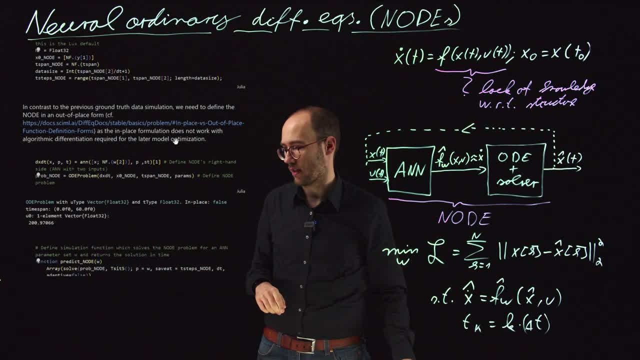 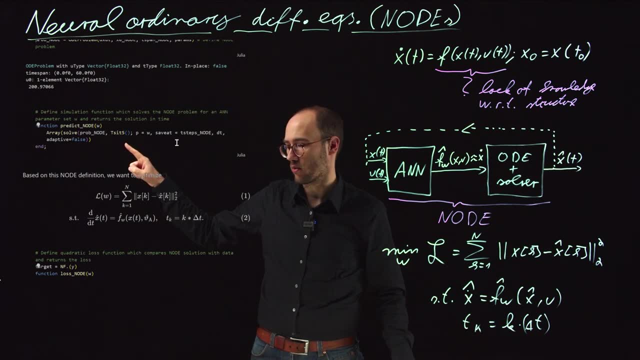 ODE problem. Of course we now need to define a cost function. for this cost function, we have predict function, which is just basically the Solve call of the ODE problem. and here's our squared loss, as already indicated here on the right-hand side for this Newton's cooling problem. 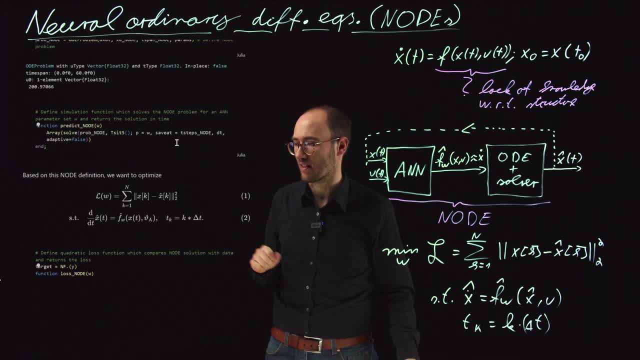 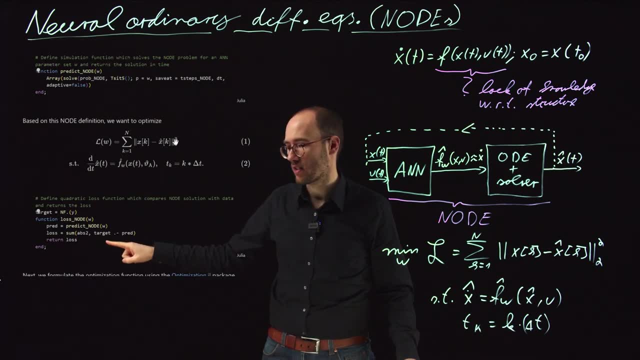 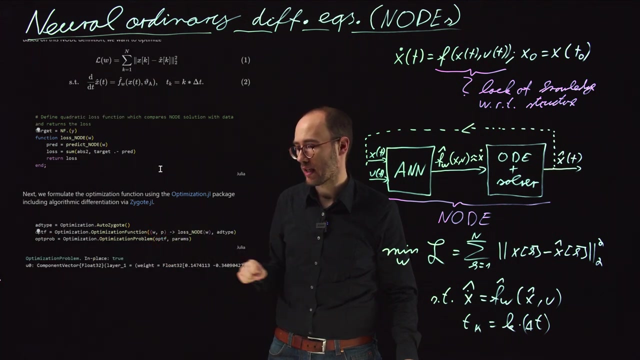 With theta a, the ambient temperature, being a constant input on the right-hand side. Then here's the loss function. straightforward, just the MSE loss targets minus predicted values Predicted this here- X hat, and the target is X, including measurement noise. If we then want to optimize that using the optimization dot JL package and with Psy code as the underlying, 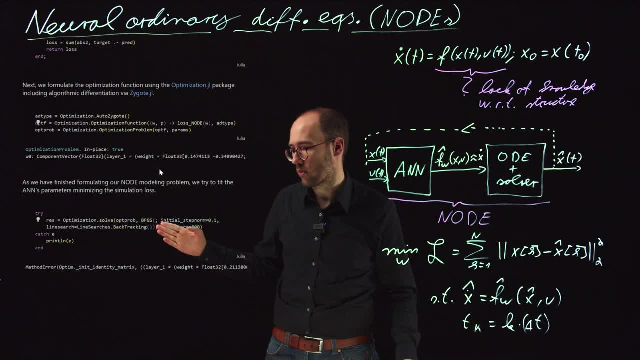 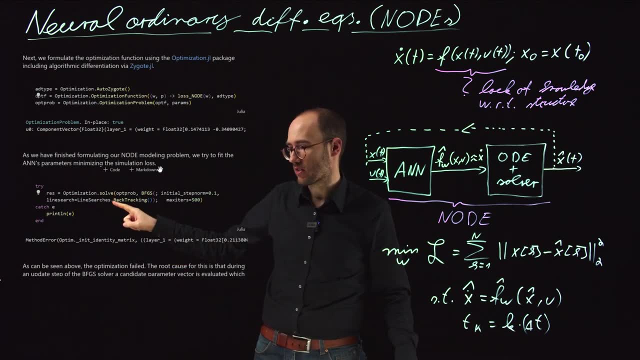 algorithmic differentiation toolbox And we start actually trying to get a solution with the BFJS solver, Then you can see with this try catch approach that actually the optimization fails, We get an error, and that it might be like a little bit confusing because this Method looks like so straightforward and if we now try to solve for the right-hand side parameters we get an issue. 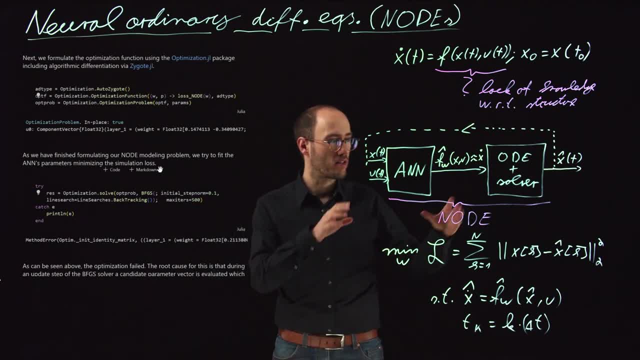 What is the root cause of that issue? the root cause of that issue is that this package of A and N ODE plus solver of course needs to be well defined, and especially if you consider the stability question, either in terms of the dynamics of the right-hand side or of the numerical point of view of the 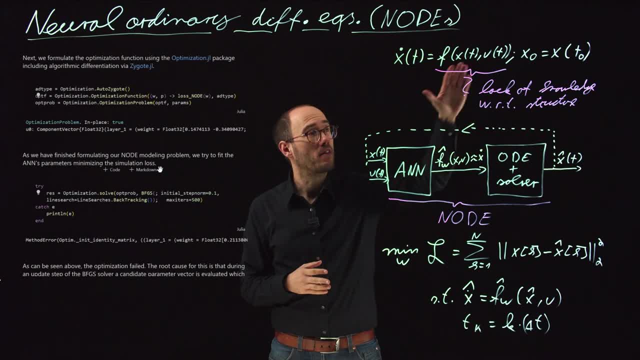 right-hand side using ODE solvers. if this right-hand side is Instable due to the actual dynamics or due to the numerics Represented by an A and N, then of course this Simulation loop crashes because the ODE solver tries to put out very, very large numbers. 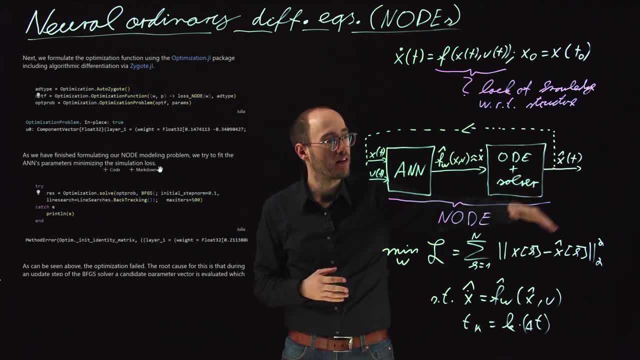 Which are numerically infeasible, and therefore, if the underlying ODE solver loop crashes, of course any optimization loop Which tries to find the best possible parameters, Metas W, will also fail, and that is actually what is happening here. We can also visualize that by utilizing not the BFJS solver. 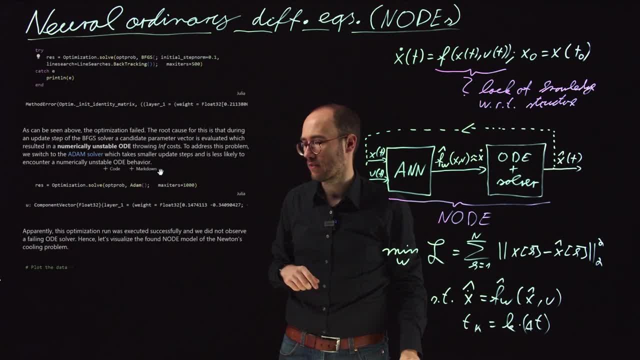 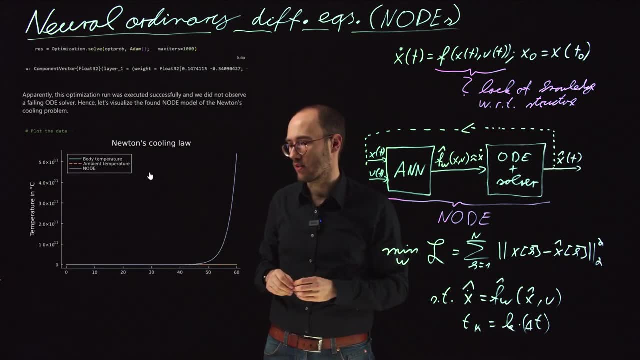 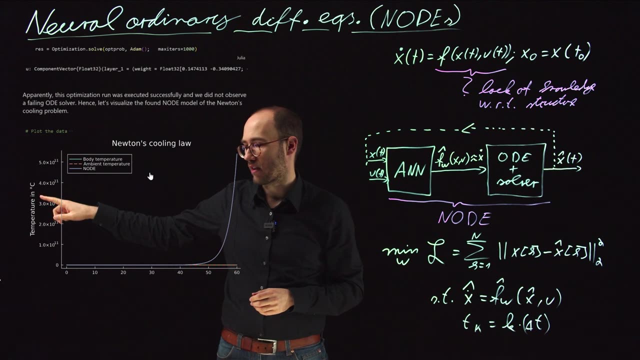 But the ADEM solver, which is a little bit more conservative, so which does not completely crash this optimization and simulation loop. But from the found result using the ADEM solver, We can already see that the node approach in this application is not successful. because if you're looking here at the temperatures, 10 to the power of, 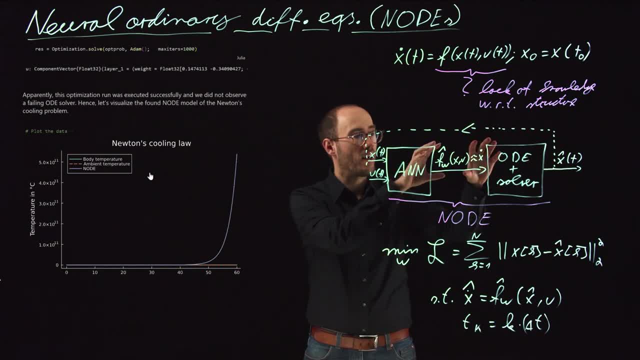 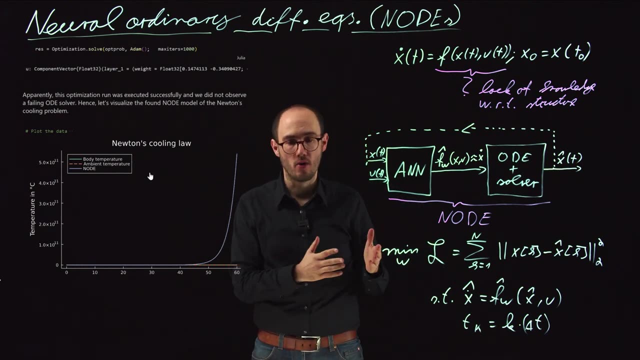 Minus 11, you can basically see that this right-hand side, represented by an artificial neural network, Went numerically instable and therefore this entire loop is not feasible. Okay, so what have we learned so far? We have learned that the node approach seems to be appealing because we do not need to apply. 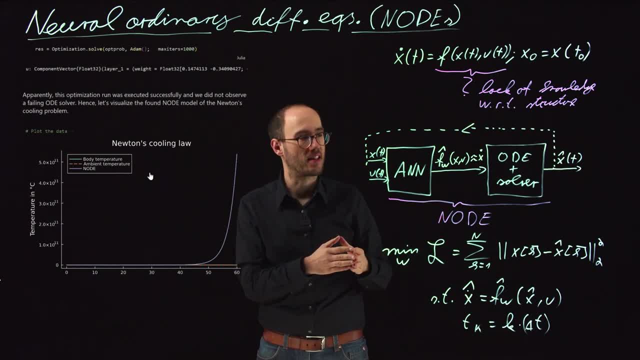 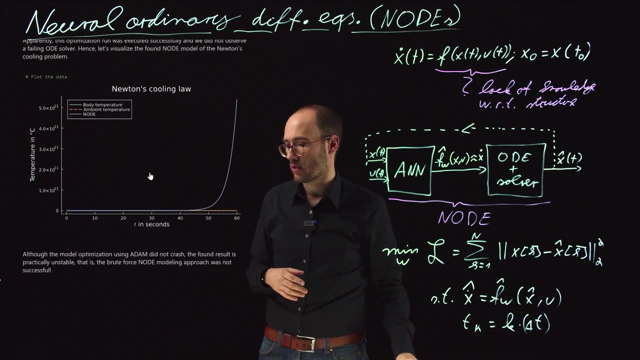 Eventually any pre-knowledge. but it can be also nasty in that thing that this simulation loop Needs to be stable. What can we do, in our example, with Newton's cooling, in order to stabilize it? I have prepared two remedies in order to do so. the first remedy is quite simple. 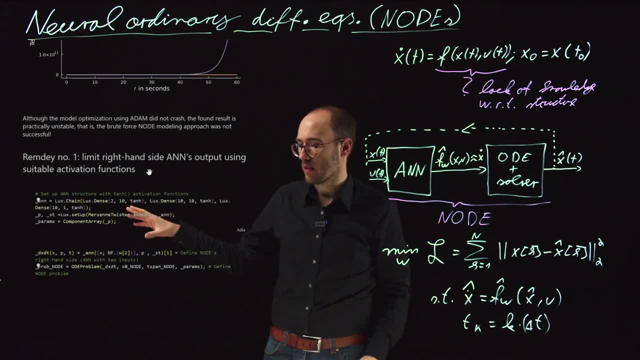 We are going to just Modify our right-hand side by adding activation functions. in particular, We are using the 10h activation function here at the input layer, at the hidden layer and specifically at the output layer. so that basically means that f hat will be limited to minus 1 and plus 1. 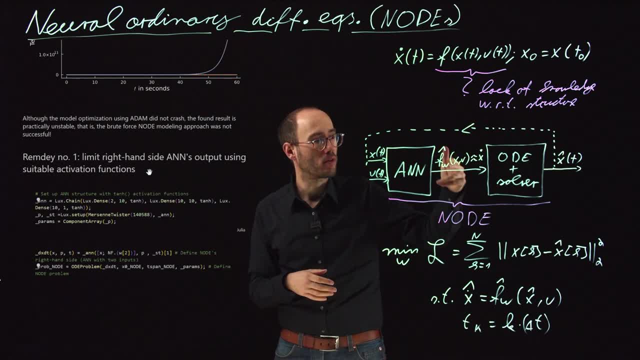 So that already limits basically the output of the right-hand side ANN and therefore this entire ODE loop gets stabilized in terms of the numerics. With this modified ANN we are basically just going through the same optimization loop as before. so we modify our ODE problem, so we take this new ANN. 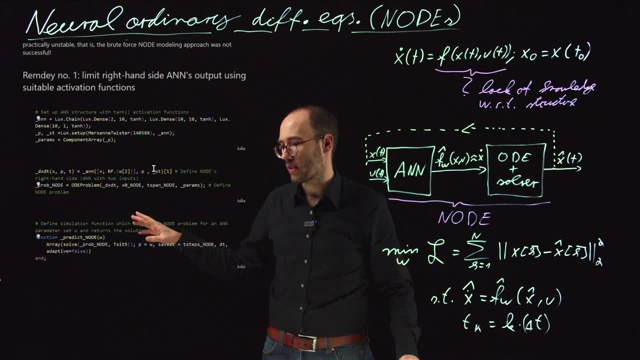 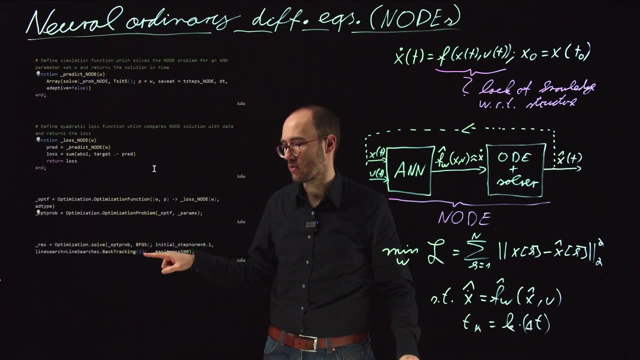 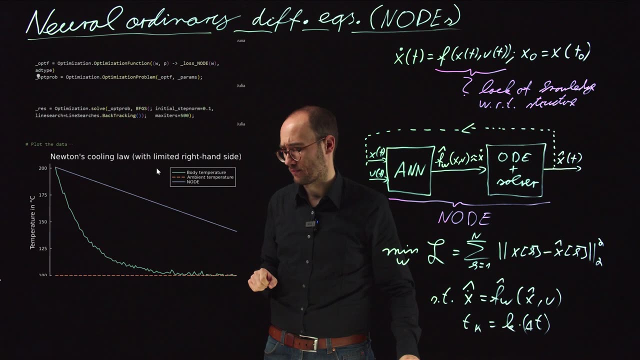 and in a new ODE problem and we put it again into our solver or ODE solver. then we put it into our loss function, we optimize it using again the BFGS solver, which completely crashed on the first attempt, and then we look at the results after solving it and what we can see from this figure. 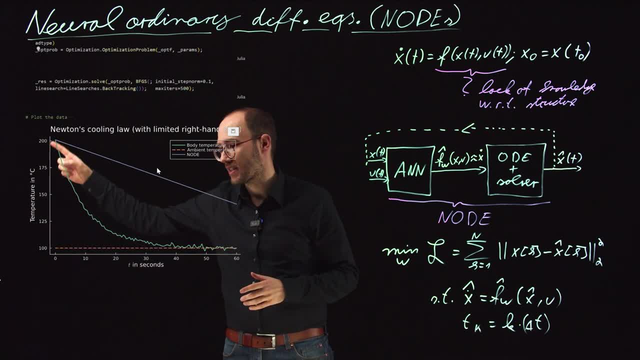 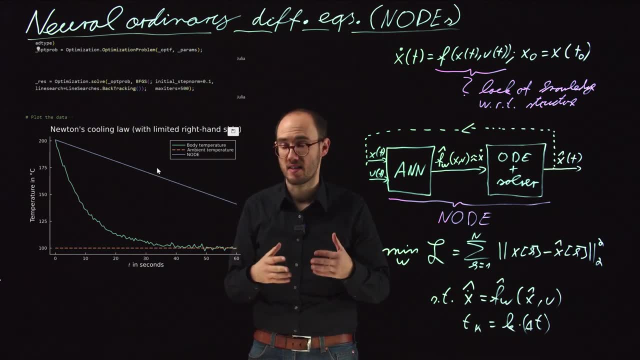 is now that eventually, if we're looking on the y-axis, the solution was successful. so if you also read out the solution printer of the optimization loop, you would see that it's actually converging into an optimum. however, due to our activation function, of course, we have also limited the 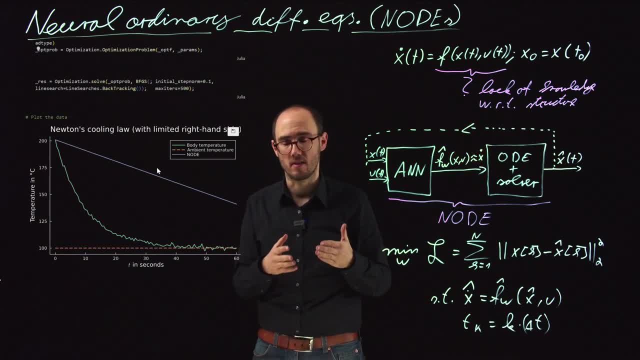 right hand side of the ODE. as I said, it is limited due to the tan h, between minus one and plus one, and if you consider that the right hand side of this ODE can be just between minus one and plus one, that of course also means that we have 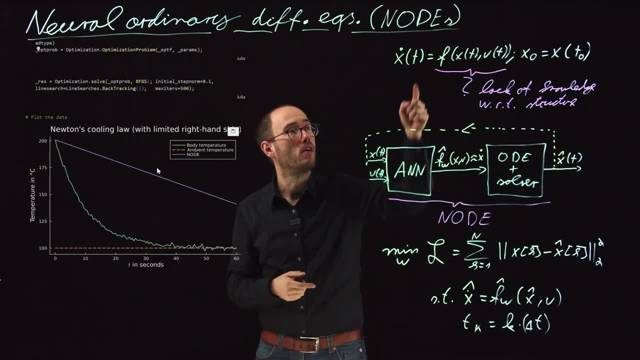 reduced or constrained the slope of x dot, and that is exactly what we can see here, because this decline, this blue line, is basically just a decline with a slope of minus one, because our activation function here, of course, limited the right hand side output, which is good in terms of the numerical 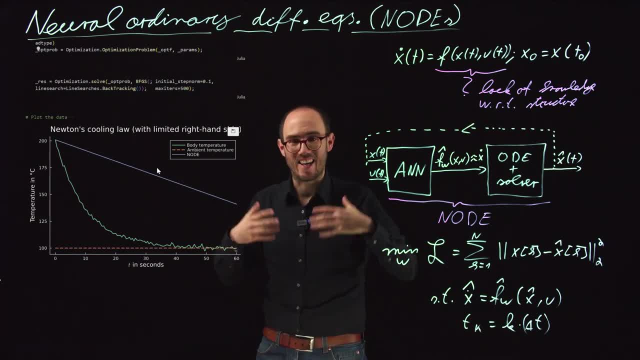 stability, but it also basically limits the dynamics which I can represent by the right hand side of this a and n. Okay, So this first remedy at least stabilized the optimization and simulation loop, which is good, but obviously we can see that the result is still not decent because we have this huge systematic error. so we need 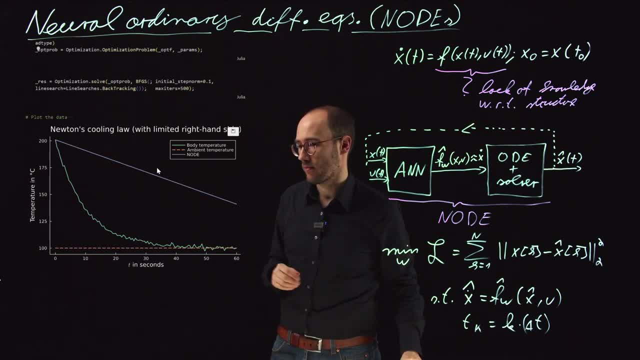 another remedy. what can we do there? of course, here we utilize an a and n based on physical data, so we see here temperatures between 100 and 200 degrees celsius and we have this tan h function in terms of the output, which is of course limiting the dynamics. so what we can actually do is we can try to. 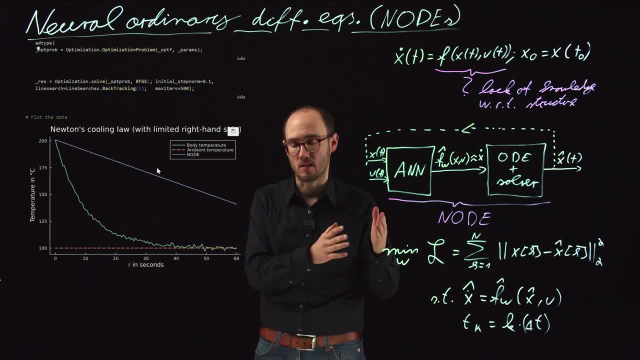 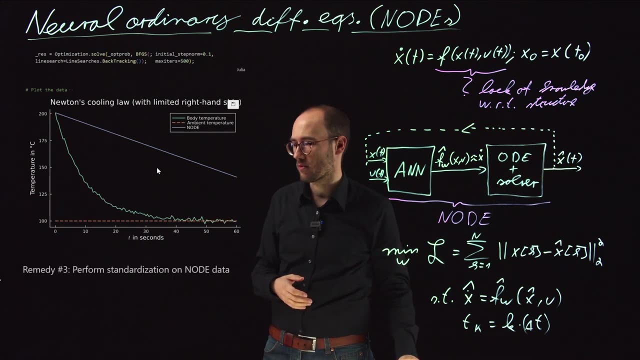 standardize the ground truth data and the input data and then utilize the a and m approach on the node context into a latent space of standardized inputs and outputs and then transform the ODE output later on. so that's the second remedy. I would like to showcase to you the performing standardization. 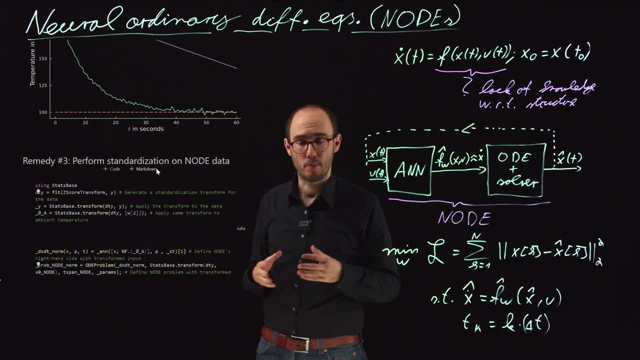 for that we are using the stats base package of Julia, which basically uses a transformation command applying the normal z transform, z score transform, which is standardization, by subtracting the mean and dividing by the standard deviation of the signal, here in particular the ground truth signal, and 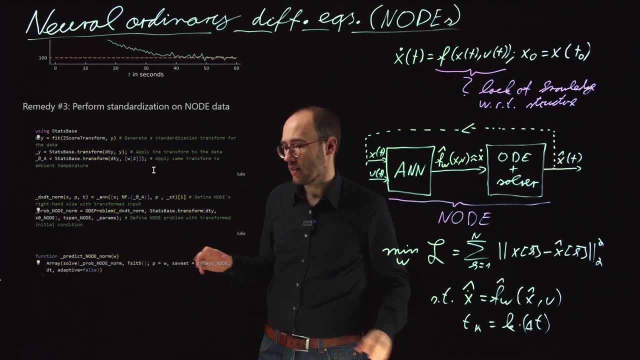 the ambient temperature. with that we utilize the same a and n structure, so we don't change something structurally on the right-hand side or the proxy of our right-hand side. the only new difference. what we do now is basically that we perform a solution based on the standardized 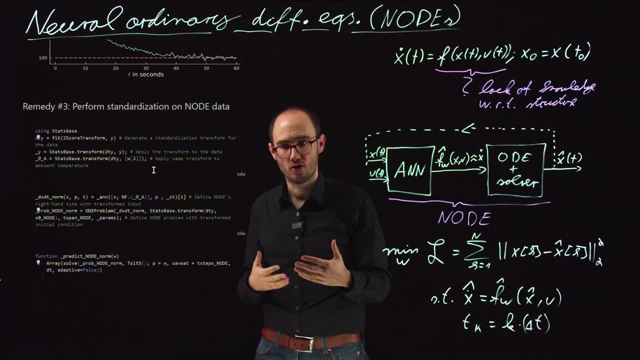 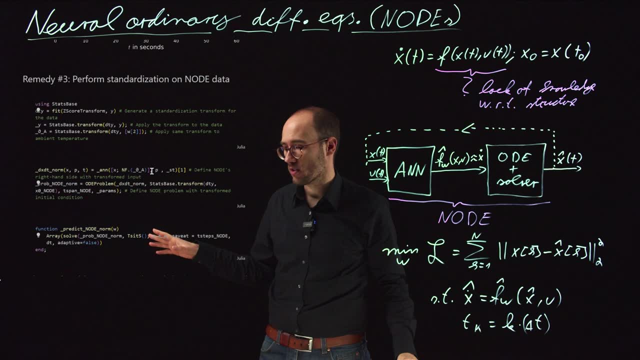 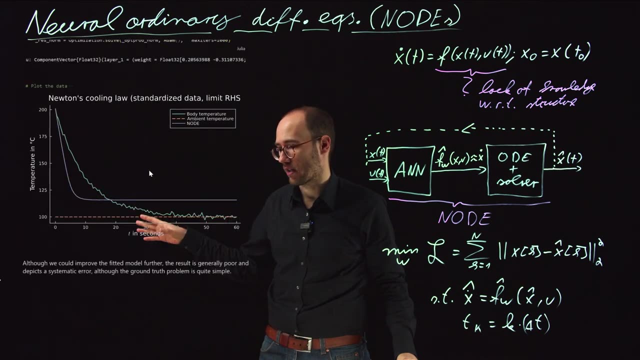 ground truth, data and inputs. so we just change the data representation, same structure of the node. so with these new data structures, we go again through the prediction, through the loss node, through the optimization loop and eventually we will plot the result, after re, of course, transforming the standardized data. 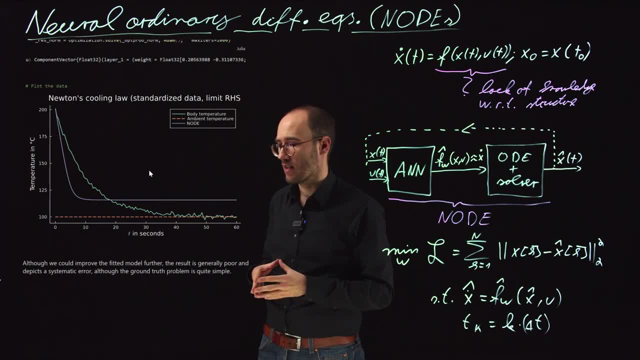 into the normal temperature and time space, and what we can see here is that the result already improved. right, so we have the blue node. response is somehow not similar, not ideal, but it goes into the right direction of representing the Newton's cooling dynamics. so that already helped. so at that.